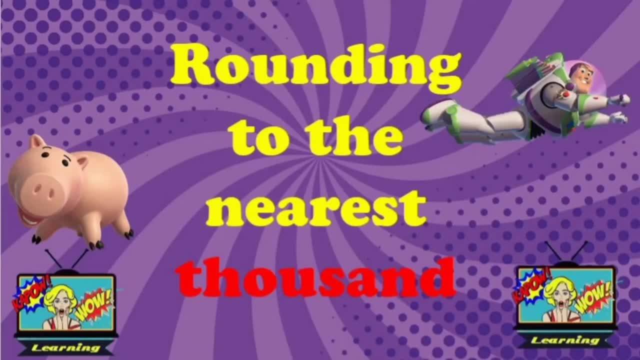 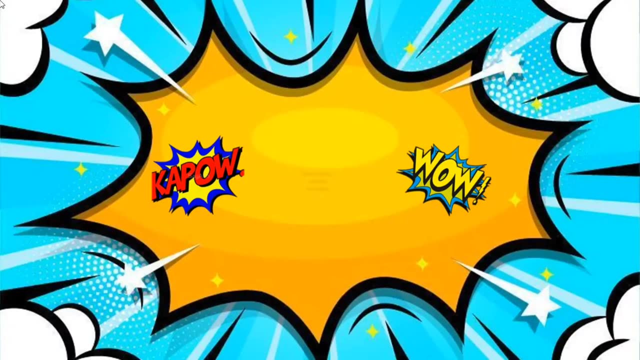 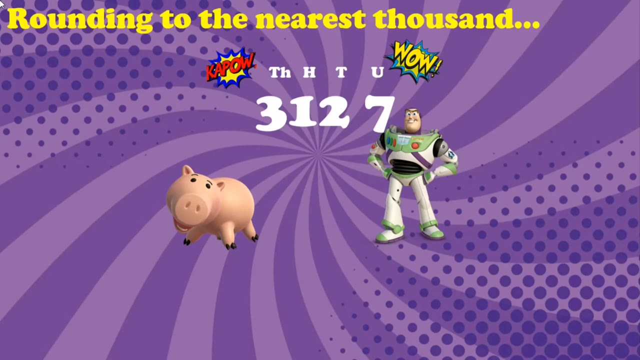 Hi there and welcome to Kapow Wow Learning, and today we're going to be looking at rounding to the nearest thousand. Okay, you can pause and play this as you watch this Rounding to the nearest thousand. So here we have number 3127.. Okay, so when rounding to the nearest thousand, we need to 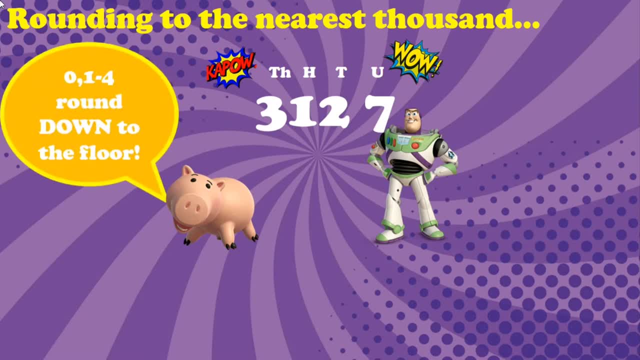 remember, all rounding 0, 1 to 4, we always round down to the floor. If the number is 5 to 9, we round up to the sky. Okay, so, rounding to the nearest thousand, we need to highlight the thousand, which is the 3.. But we look at the number before, which is the hundredth. Now the hundredth is a 1.. So 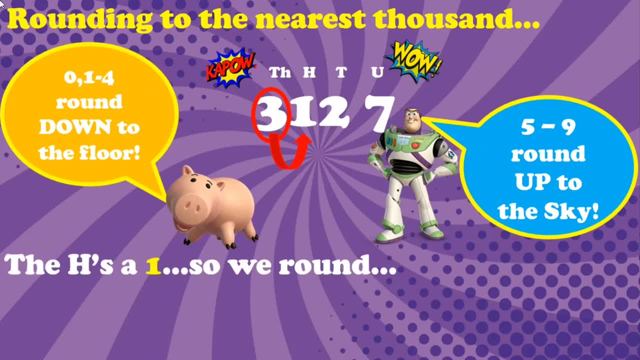 the hundredth is a 1.. So do we round down to the floor or do we round up to the sky? 0, 1 to 4. round down to the floor. 5 to 9: round up to the sky. Well, we round down to the floor. So if we round that down, your answer should have been 3,000.. 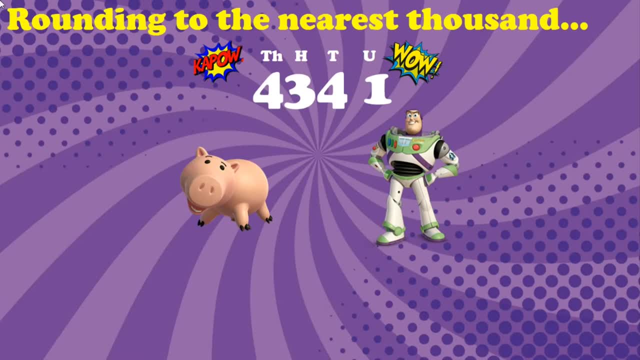 Excellent, Let's do this one. 4341.. Round it to the nearest thousand. You can pause and then play, but remember: 0. 1 to 4: we round down to the floor. 5 to 9: we round up to the sky. So pause and then. 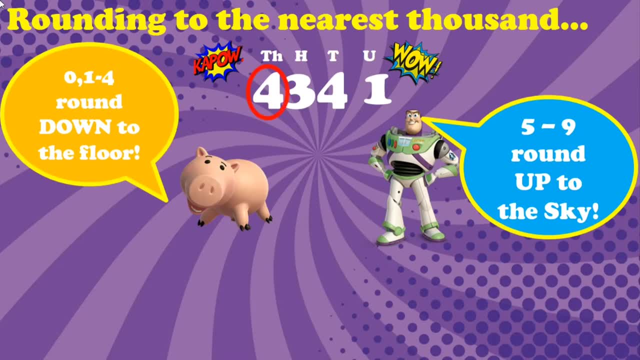 play. You should have said, Well, we sign up to the sky, We round up to the sky. So we round up to the sky. I finished, I'm in, I'm empowered. If they said: that sounds great, cool, If they. 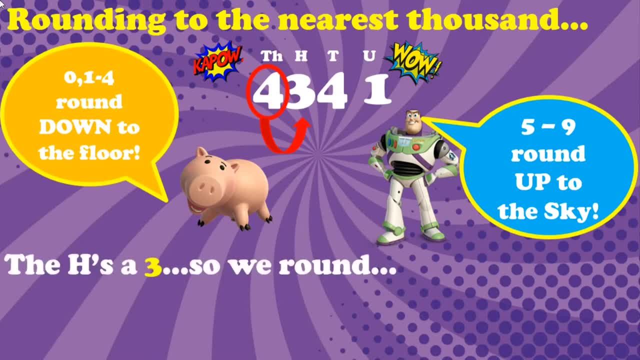 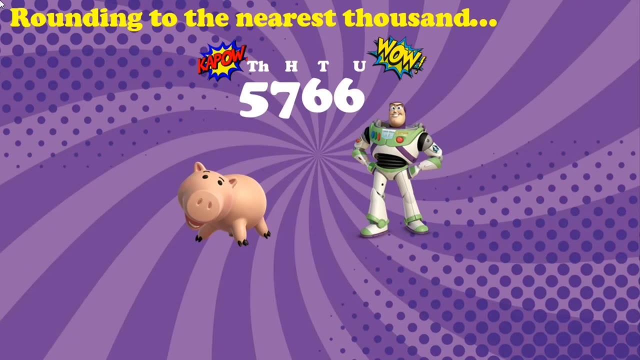 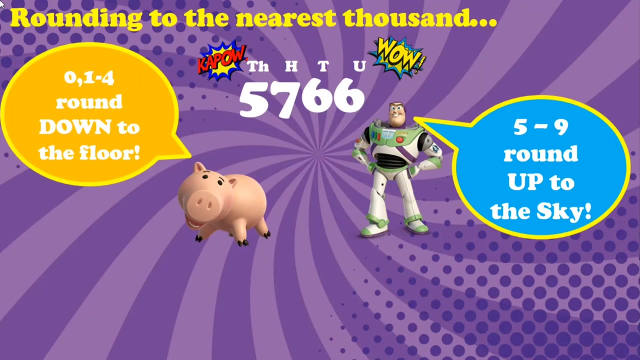 even said it says that it's too fun if they do it anyway. put away all the thoughts in the Q. We should find out how to figure out how to figure that- probably one of the last questions. Animal R propose Sonata kata, kata or we round up to the sky. so remember, you can pause and then play it right. here we go, so we should. 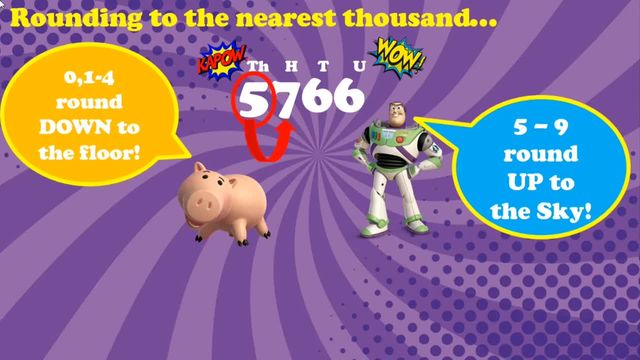 have circled the thousand. but we'll look, always look, at number four, which is the seven. so the hundreds has a seven. so we round up or down. do we round down to the floor or up to the sky? you should have said up to the sky. so the next thousand after five thousand is six thousand.